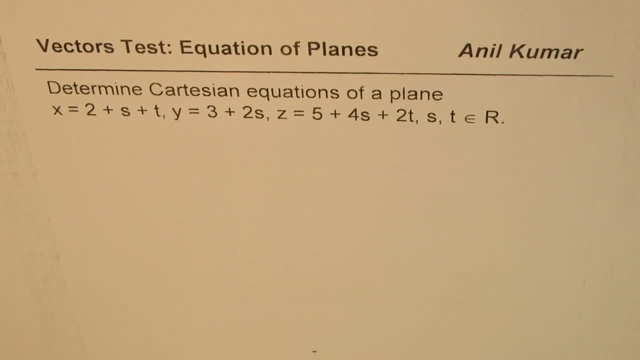 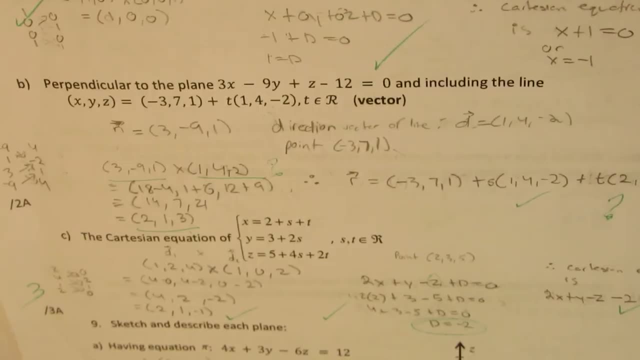 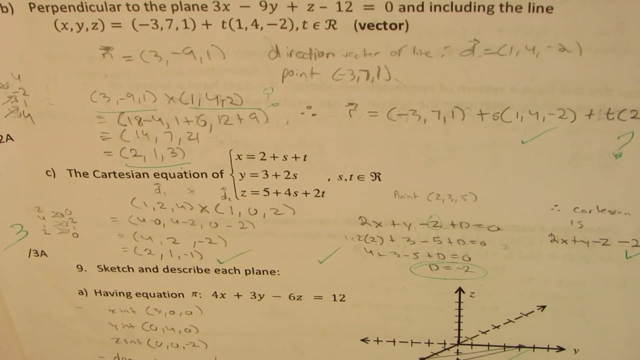 I'm Anil Kumar discussing with you previous test paper questions on vectors equations of plane. Now I'm taking up question number 8, part C, where we'll write: we'll find Cartesian equation from given set of parametric equations, right? So the question here is: 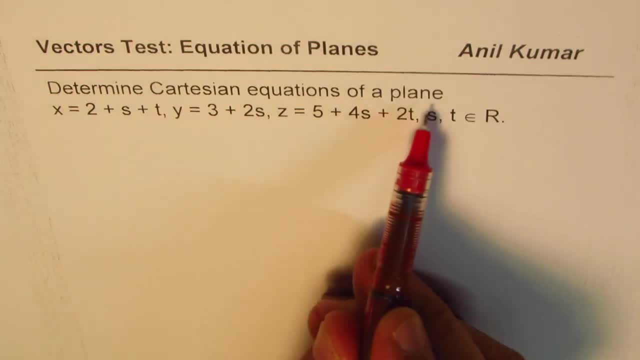 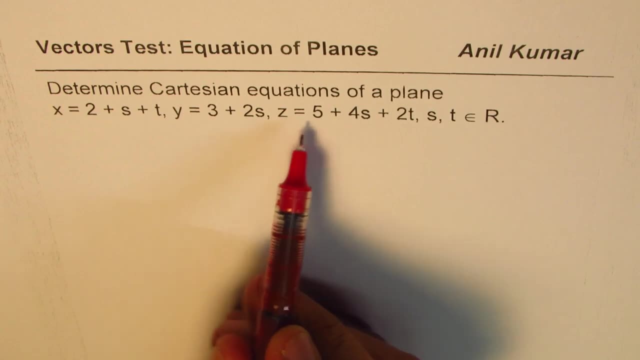 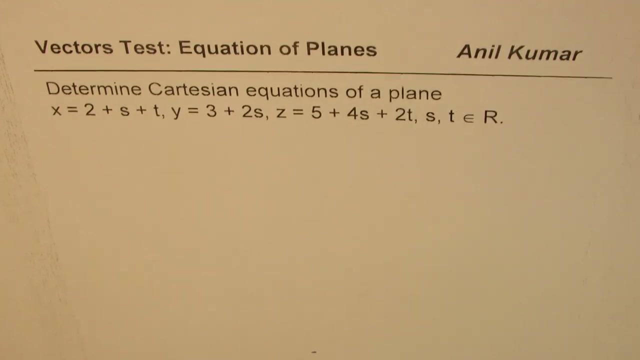 determine Cartesian equation of a plane where x equals to 2 plus s plus t, y equals to 3 plus 2s, z equals to 5 plus 4s plus 2t, where s and t belongs to the set of real numbers right. 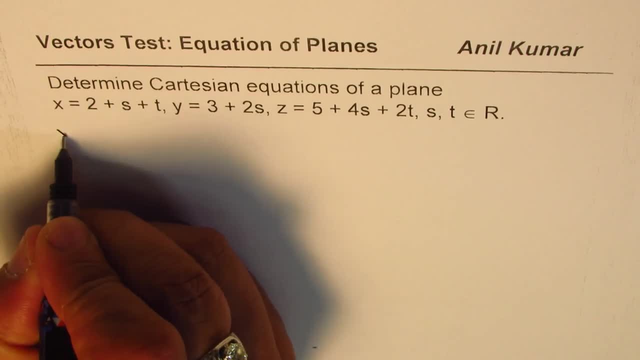 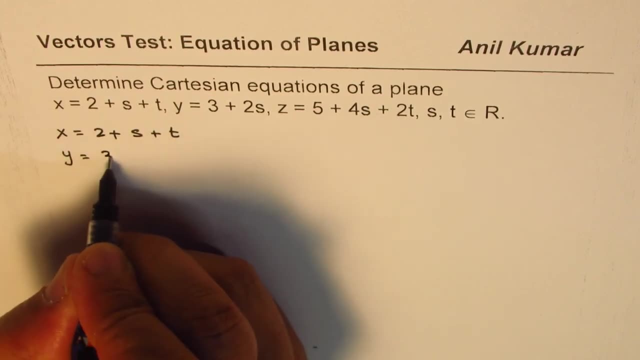 Now from these equations, let me rewrite them. So we are given: x equals to 2 plus s plus t, y equals to 3 plus 2s, right? So there's nothing in t. So let me write here: 0t, okay, And z equals to: 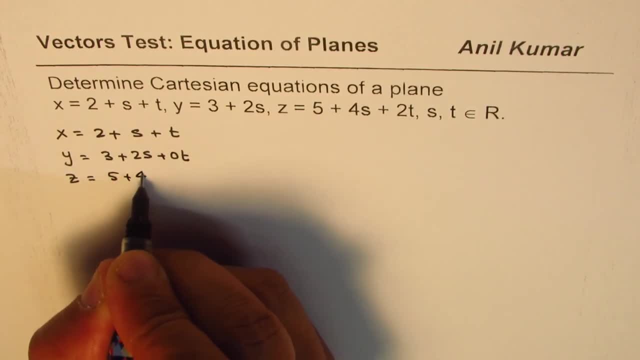 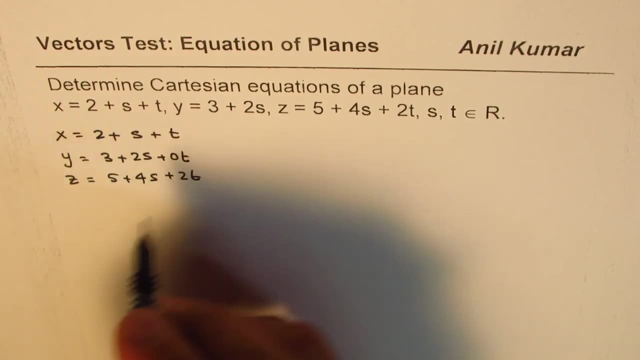 5 plus 4s, 5 plus 4s plus 2t. right Now, from this information, what do you get? You get a point. so you get a point P which is, let's say, 2,, 3,, 5.. 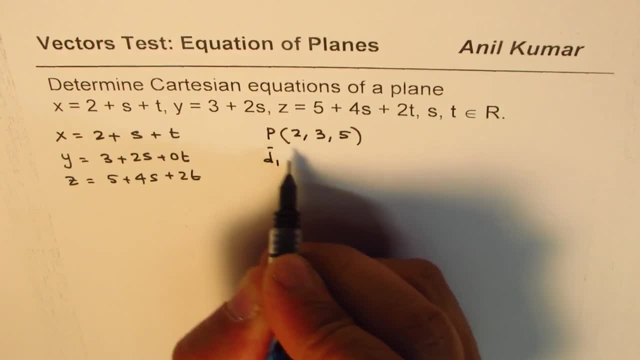 You get one direction, d1,, let's say, which is 1, 2, 4, right, 1, 2, 4.. And you get another direction, which is 1, 0, 2, 1, 0, 2,. okay, All this information. 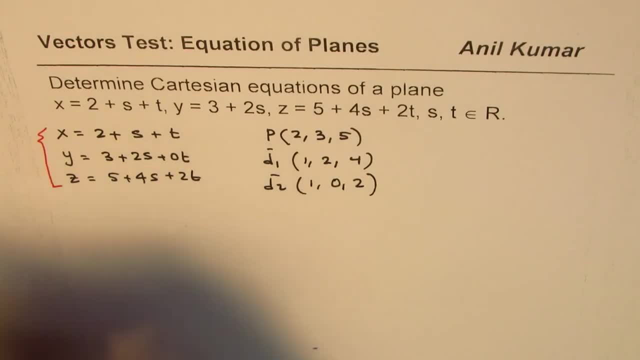 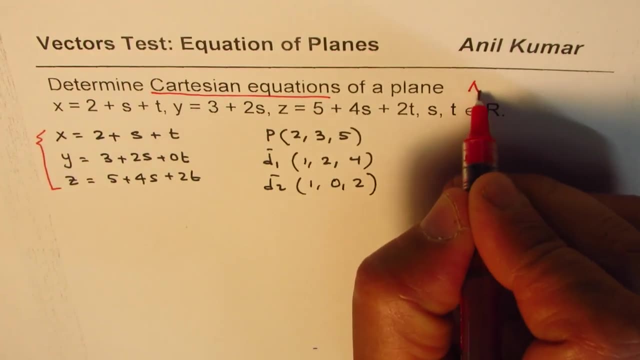 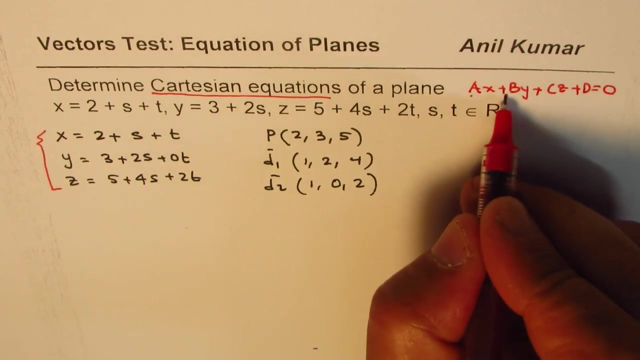 you get from this parametric set of equations. I hope that point is clear. Now we need to write the Cartesian equation, which is of the form: ax plus py plus cz plus d equals to 0, where abc are normal vectors, right. 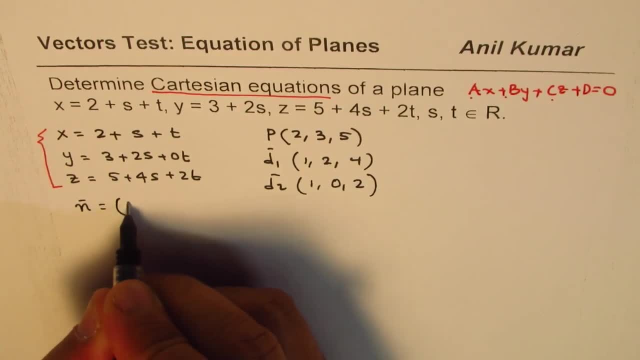 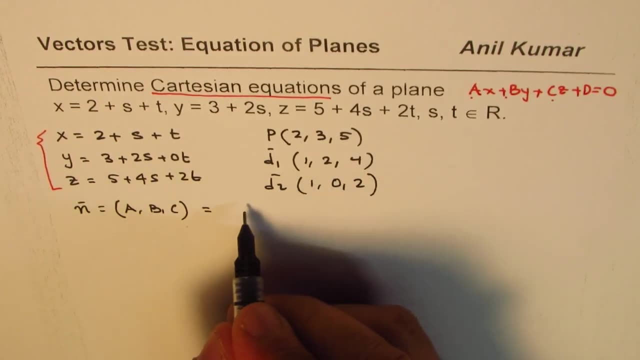 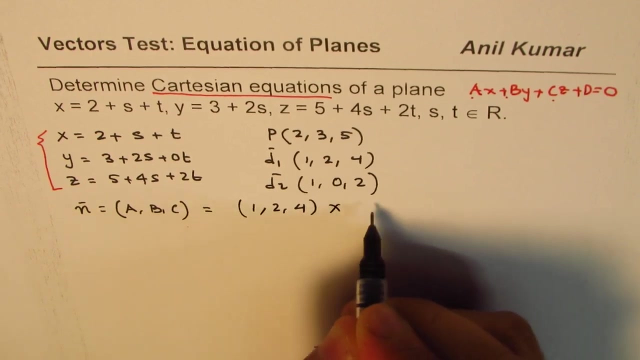 So we are saying: normal is abc, is it okay? And how do you get them? You get them by cross product of these two, So you can do d1 cross d2, or let me write 1, 2, 4 cross 1, 0, 2,. 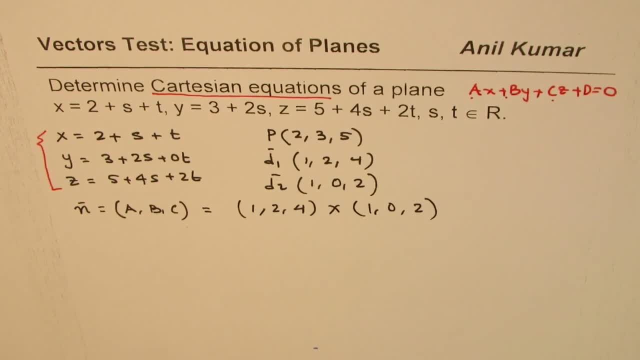 right. So that is how you get your normal vector right. So let me do this cross product using the method of matrix. So we'll use, let me say, 1, 2, 4, 1, 2, 4,, 1, 2, 4, 1, 2,. 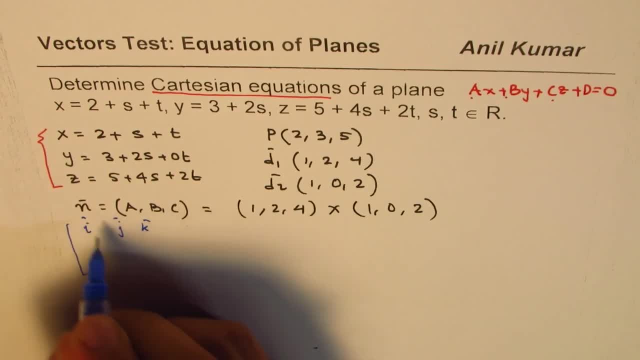 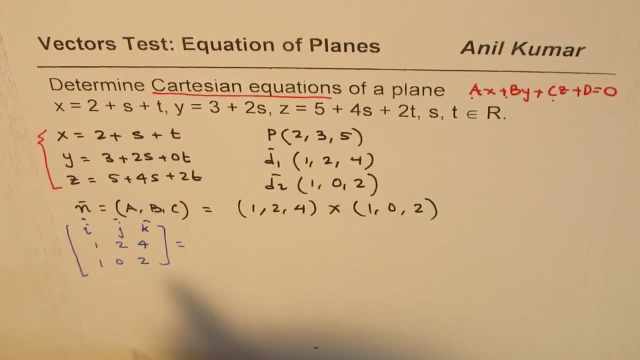 say i, j, k unit vectors along x, y, z, 1,, 2, 4, and 1, 0, 2, okay. So that gives us: i times 4 minus 0 minus j, times 2 minus 4 plus k, times 0 minus 2, okay, And that gives. 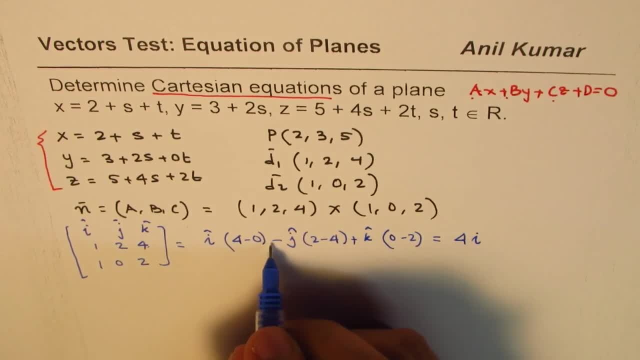 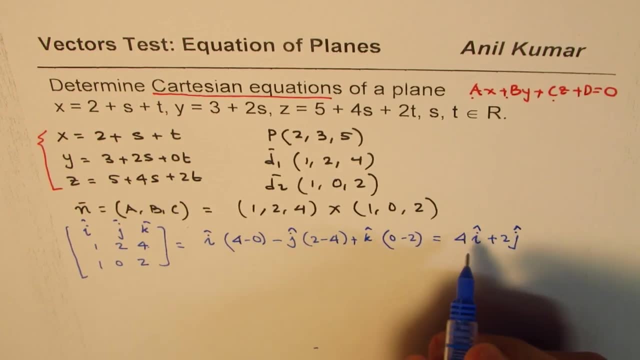 you 4i Minus. this minus minus becomes positive, so positive 2j. these are unit vectors, right? So we put this kind of a symbol here and there is minus 2k, So that is the normal vector. 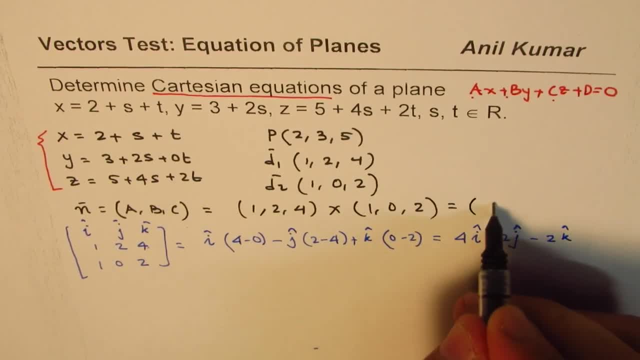 right. So the normal vector which you are getting here is 4, 2, minus 2, right. 4, 2, minus 2, which you could also factor out 2 and write this as 2, 1, minus 1, that's. 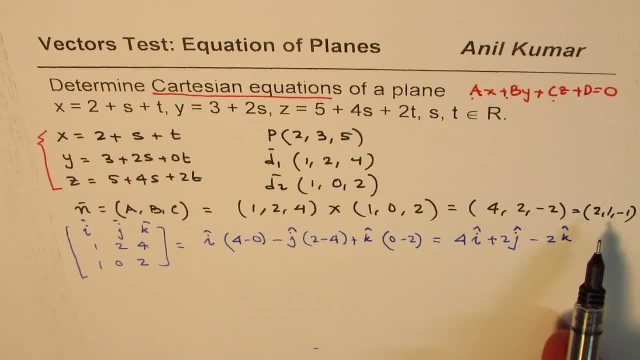 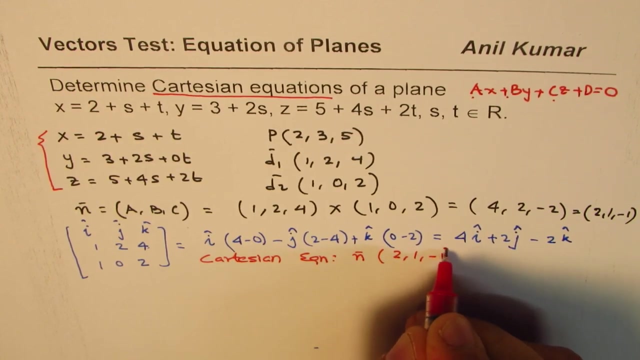 okay, Both are same, right. So that becomes the normal vector. Using this in your equation, you can write your equation as now. let me write it on the Cartesian equation now, where what we know is that the normal vector is 2, 1, minus 1, and the point P is 2, 3, 5,. 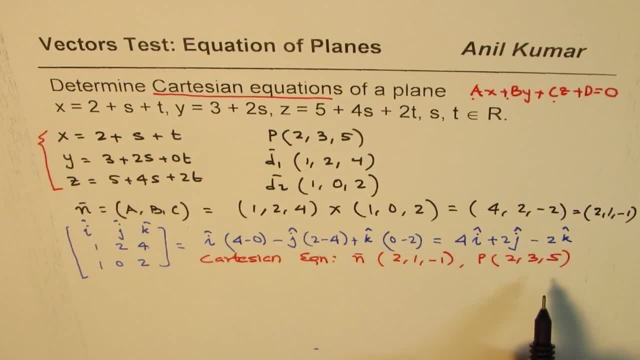 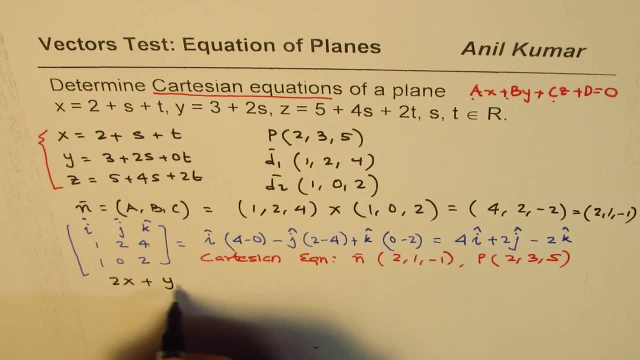 right, Okay, So you can actually pause the video. do this part on your own and then check with my solution, So that becomes 2x plus y minus z plus d equals to 0.. When I substitute the point, I get 2. 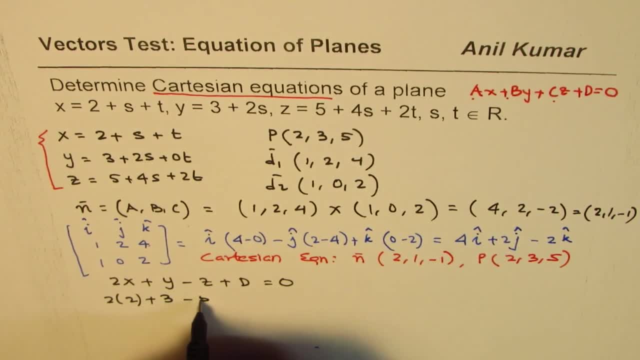 times 2 plus 3 minus 5 plus d equals to 0, and that is 4 plus 3 minus 5 plus d equals to 0, or d equals to well, we can add that 7 minus this is 2.. 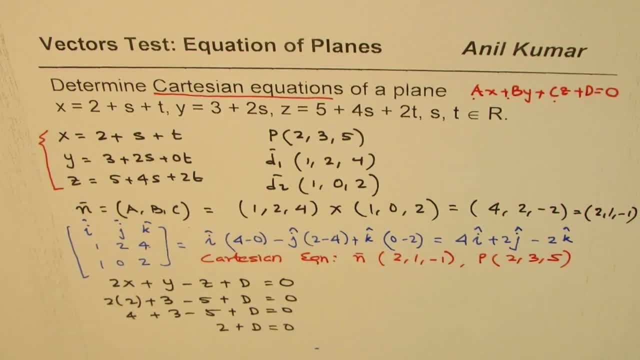 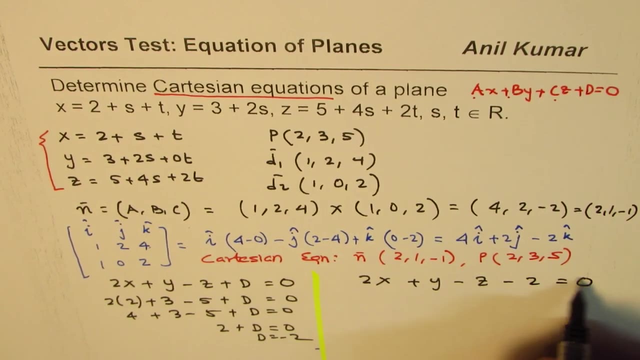 Okay, So from here you get d as minus 2, right? So the Cartesian equation is: 2x plus y minus z minus 2 equals to 0.. Is that okay? So that becomes the Cartesian equation for the given set of parametric equations.